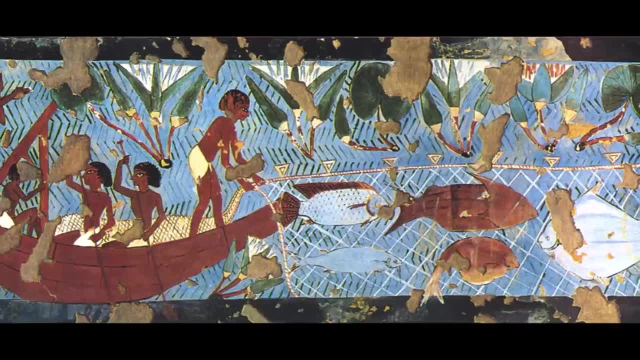 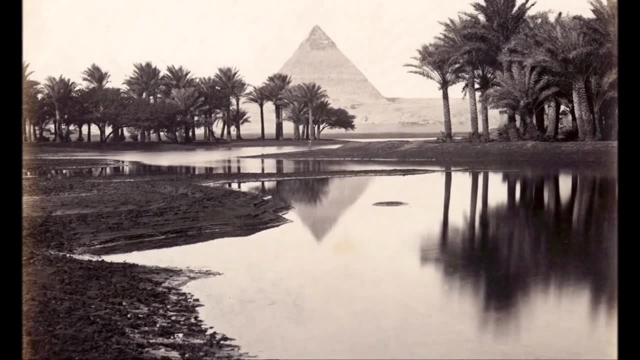 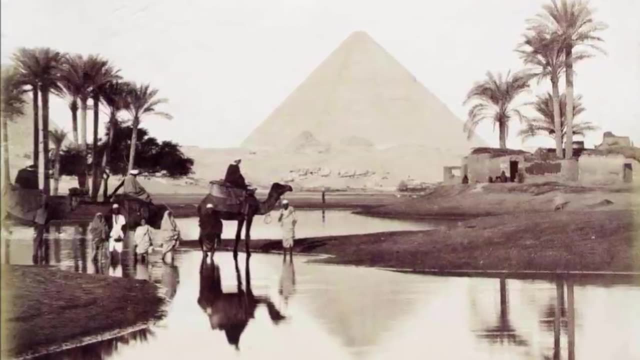 The Nile River provided the Egyptians with precious water, but also something else just as important – mud Mud. Every year, between June and September, the Nile River overflowed its banks, flooding the land on either side. But this annual flood was not a disaster: The people of Egypt. 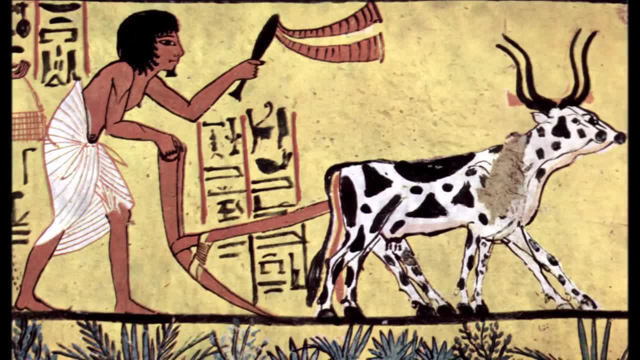 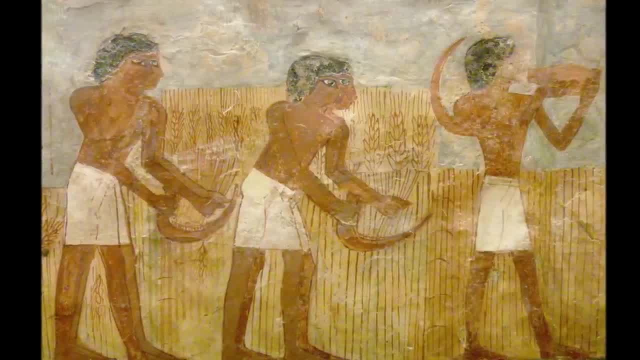 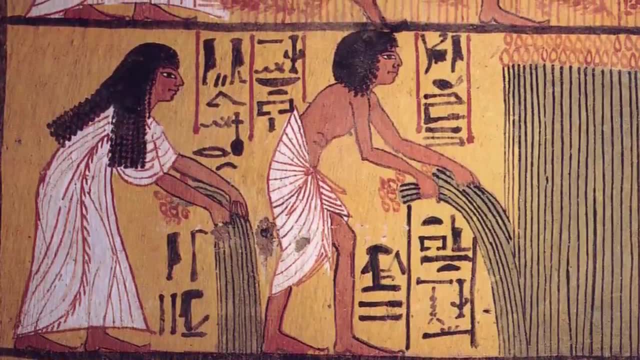 looked forward to it. When the Nile flooded, it covered the fields on both sides with a layer of rich brown mud that could grow wheat, barley and vegetables. When the river did not flood very much, the people would not be able to grow enough food. 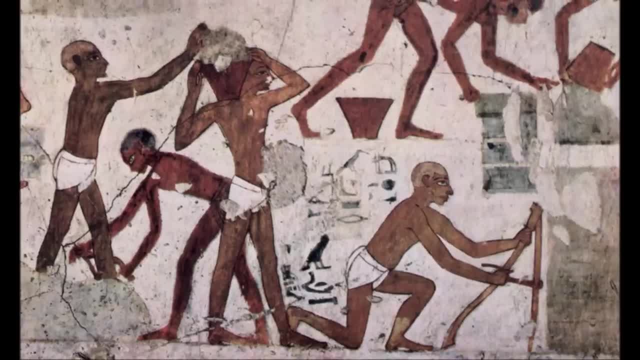 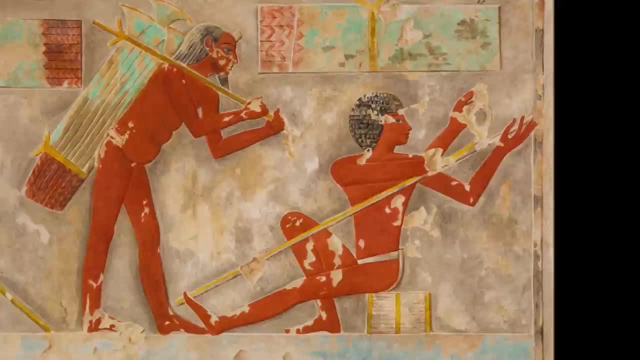 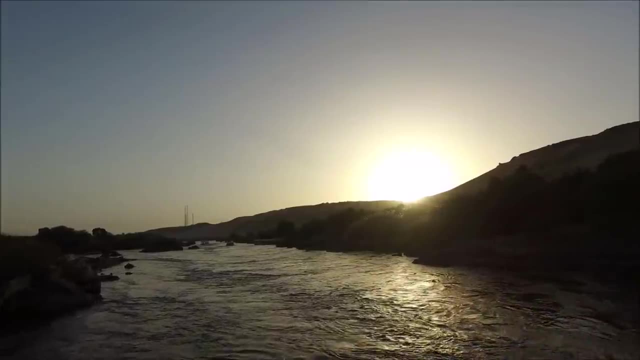 The Nile River provided other important resources as well. Mud from the riverbanks was used to make bricks. Papyrus plants growing along its edge were used to make paper baskets, rope and sandals. Even the water itself formed a sort of highway, allowing boats to transport. 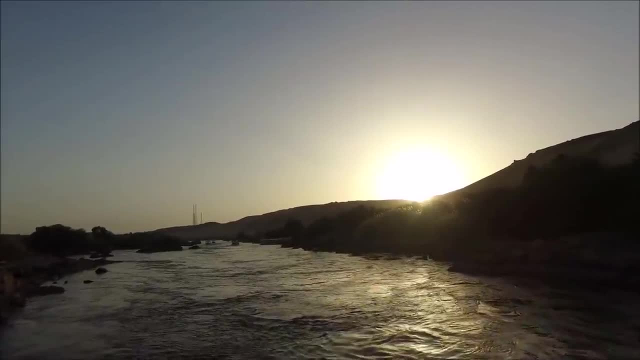 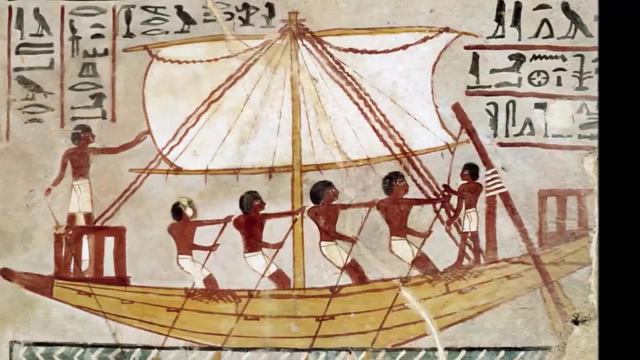 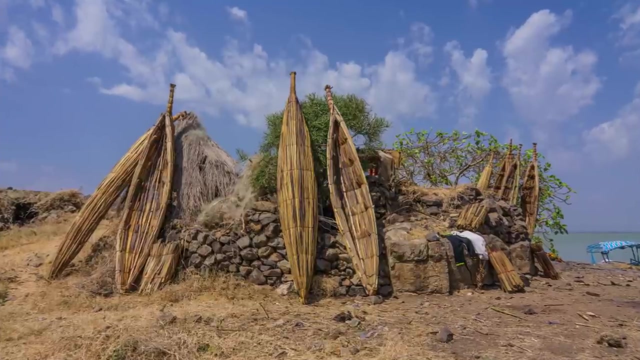 people and goods from one end of the kingdom to the other. Because of the Nile, the Egyptians became ship builders. Their earliest ships were skiffs made of bundles of papyrus reeds tied together. Air trapped in the hollow reeds helped these skiffs to float. The Egyptians would use long poles to push these early boats. 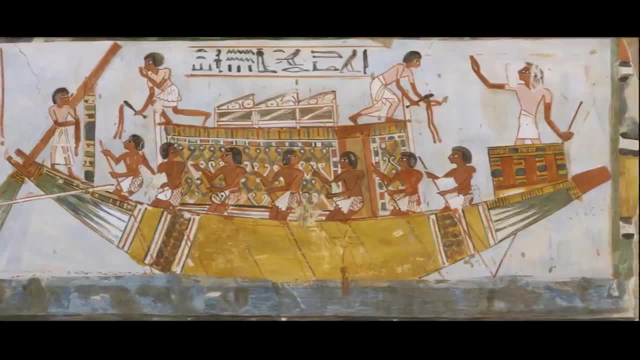 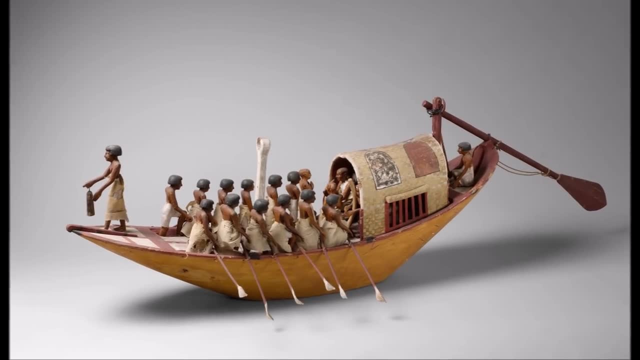 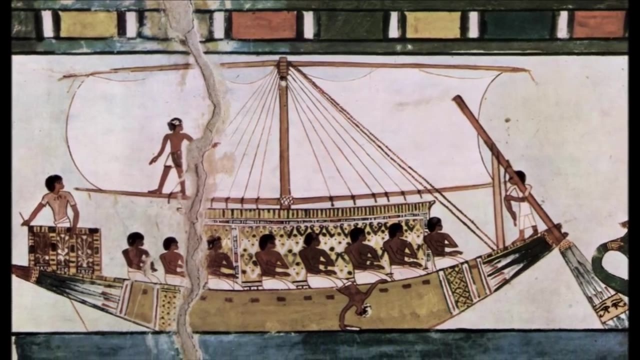 across the river. Later, ships were made of wooden planks with reeds stuffed into the cracks. At first they rowed, but later developed sails to allow the wind to blow their ships up and down the river. With these ships, the ancient Egyptians were able to trade with other countries around. 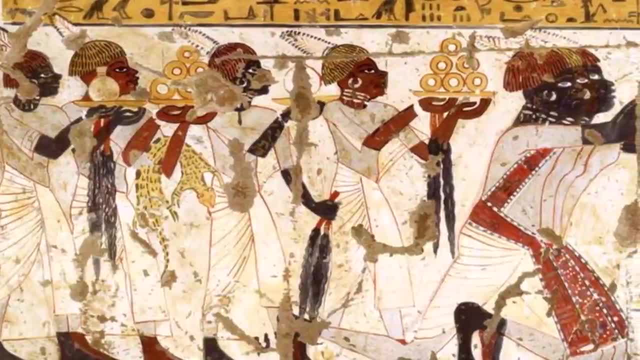 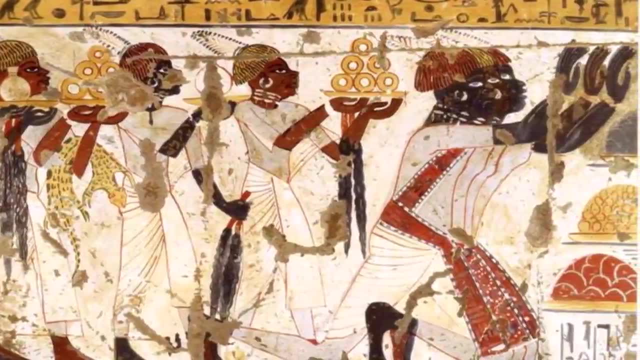 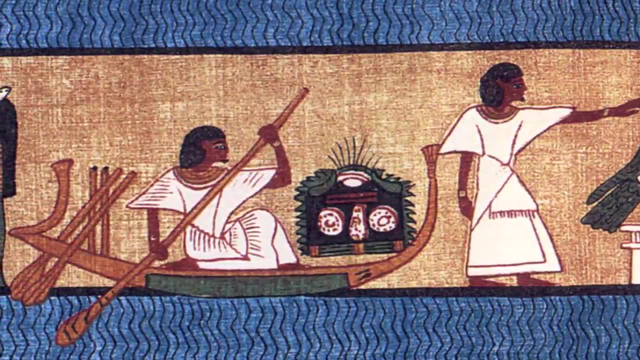 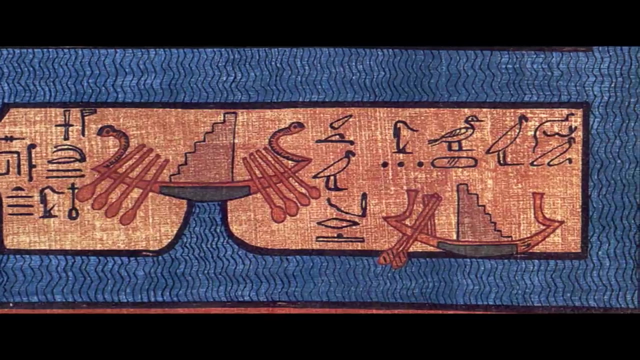 the Mediterranean Sea. They also became explorers traveling as far as the east coast of Africa and crossing the Indian Ocean. The Nile River was so important to the people of ancient Egypt that their calendar was based on it. They divided the year into three seasons: inundation, when the Nile would flood. growing. 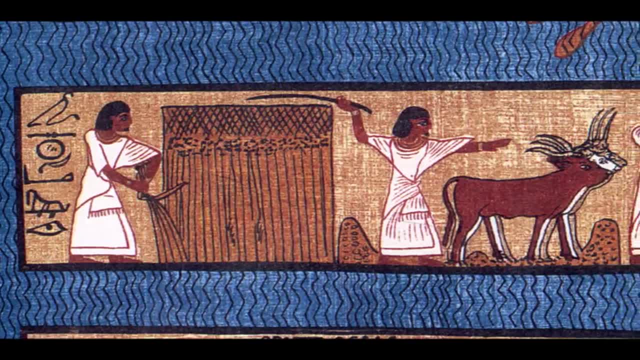 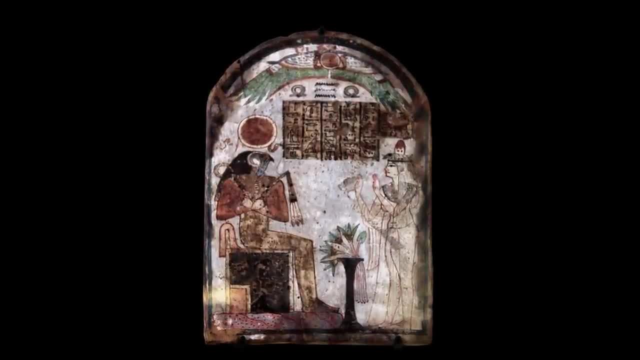 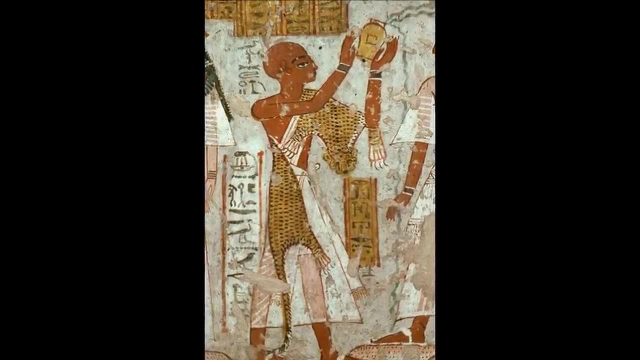 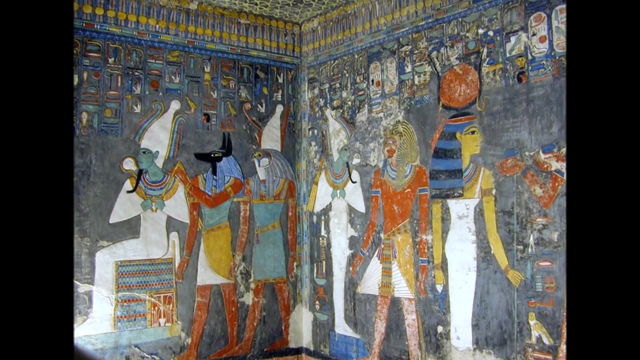 when it was time to plant crops and harvest. When things went wrong, such as the Nile floodwaters not rising high enough, the Egyptians thought it was because the gods were displeased. The people would perform rituals and make offerings to try and persuade the gods to put things back the way they should be. 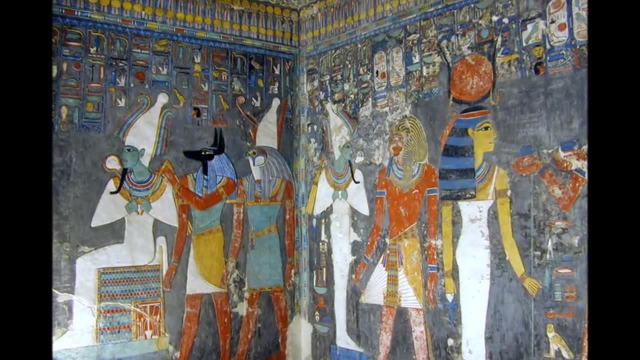 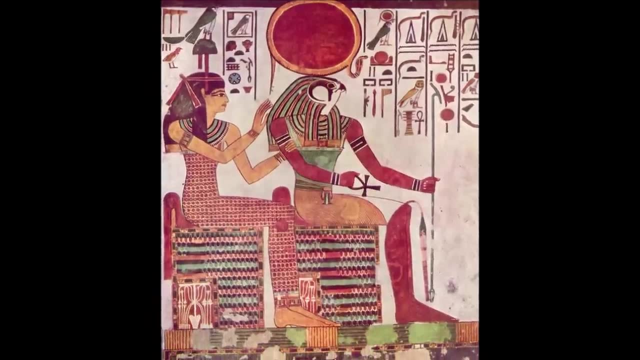 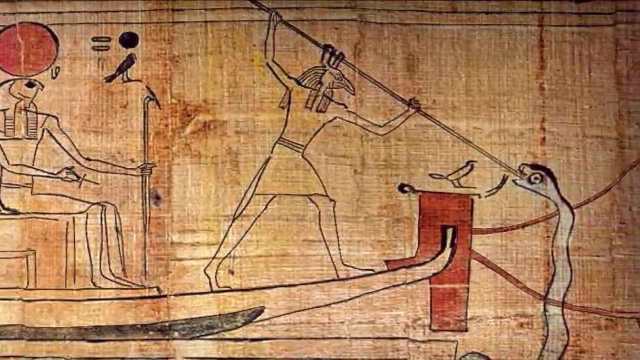 The ancient Egyptians had a god for almost everything, as many as 2,000 of them. There was a god of the underworld, of the sun, of the sky, of deserts and, of course, a god of the Nile River. 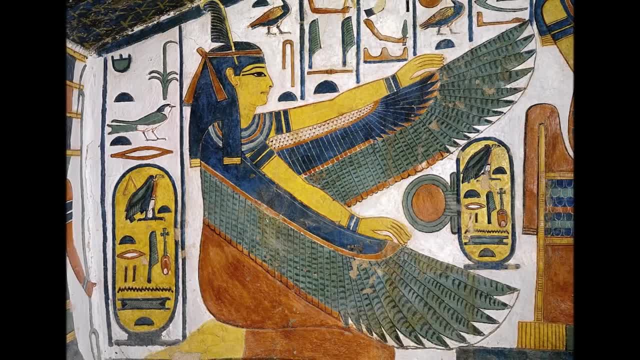 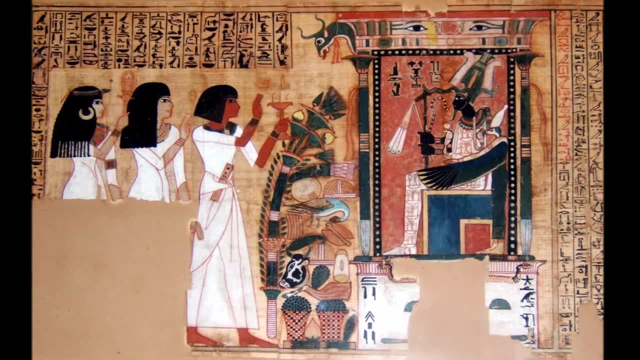 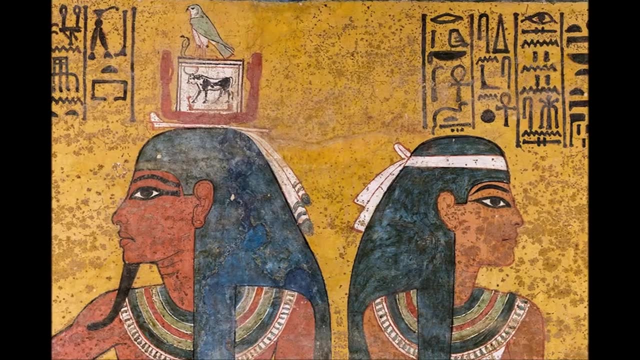 The Egyptian gods could take many forms, Often animals, and were sometimes depicted as a person with an animal's head. One of the most important of their gods was Osiris, god of the underworld. In Egyptian mythology, Osiris was a king ruling as lord of the earth with Isis, the 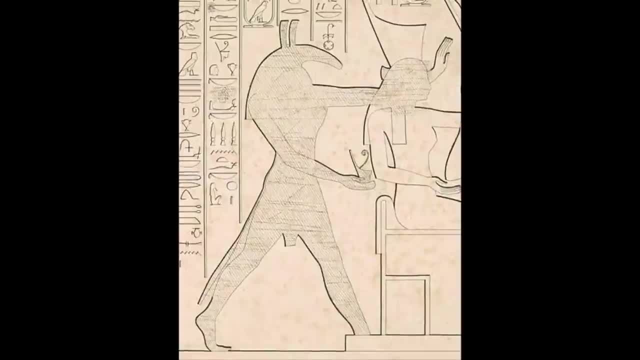 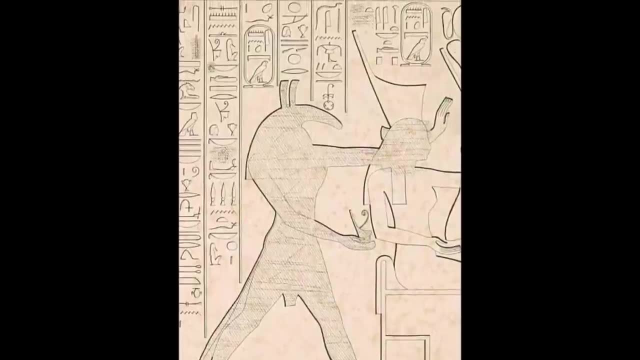 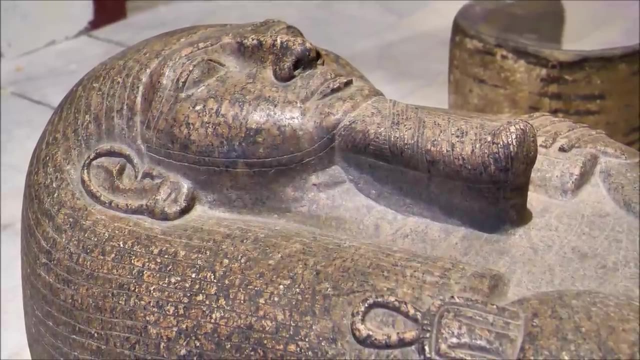 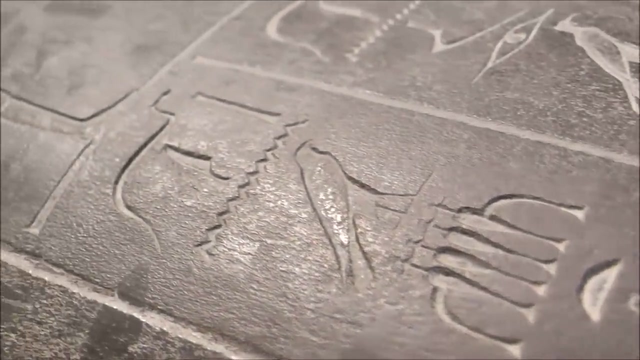 mother goddess as his queen. His brother, Set, became jealous of Osiris and came up with a plan to kill him. Set had a beautiful coffin made that was just the right size for Osiris, and then threw a big party. He told his guests that whoever fit the coffin best would get it as a gift. 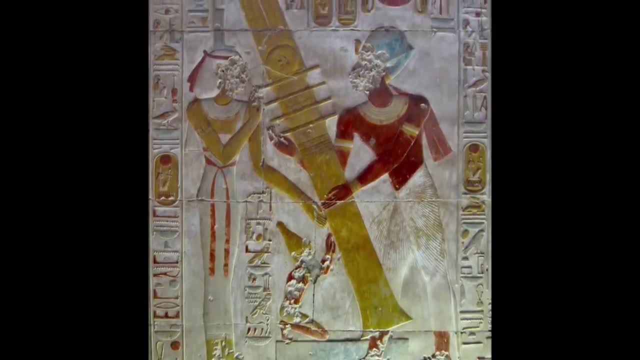 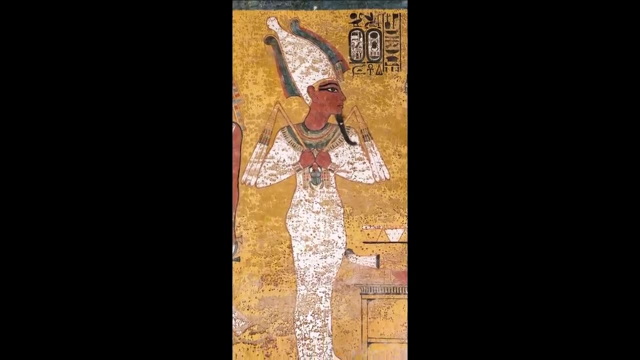 When Osiris laid in the box Set, closed the lid, fastened it and threw it in the Nile. Osiris died, but eventually Isis found his body. She was about to use a magic potion to resurrect him when Osiris was dead. Osiris died, but eventually Isis found his body. She was about to use a magic potion to resurrect him when Osiris was dead. 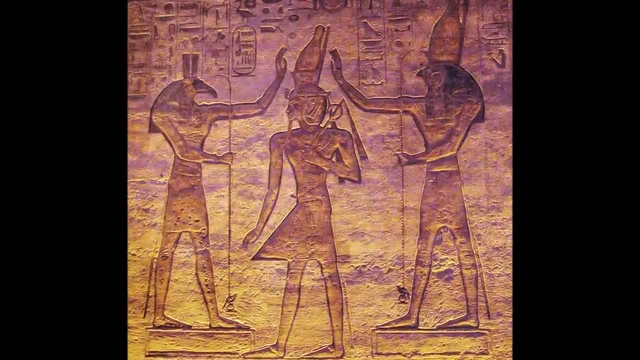 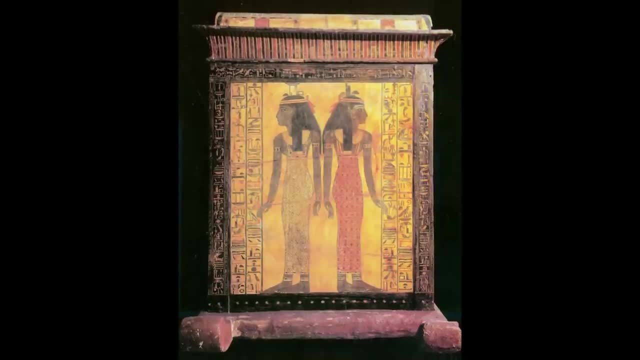 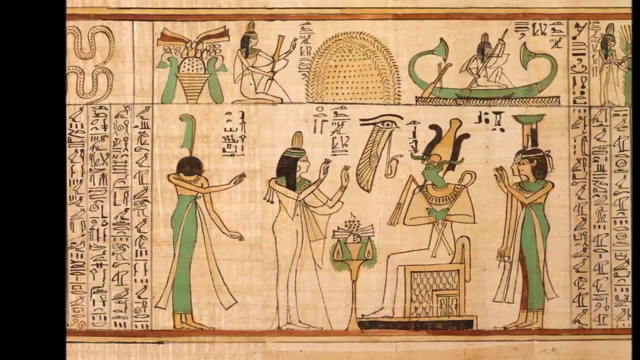 When Set cut the body into pieces and scattered them around Egypt. With the help of her sister, Isis found all of the body parts but one and put Osiris back together Because a piece was missing. Osiris could not be brought back to life. Instead, he went. 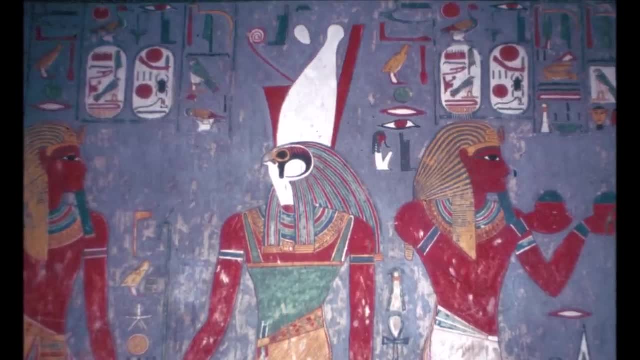 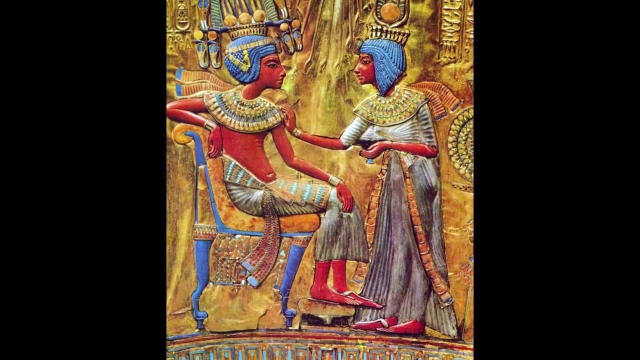 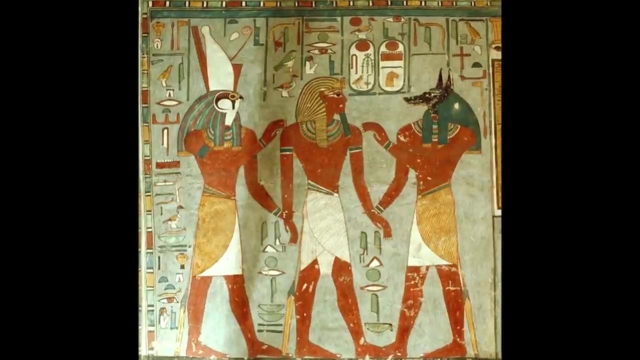 to the afterlife and became lord of the dead. Horus, the son of Isis and Osiris, became the next king. This story helps explain how the Egyptians viewed their pharaohs. Pharaohs served as rulers in ancient Egypt, but these kings and queens were believed to. 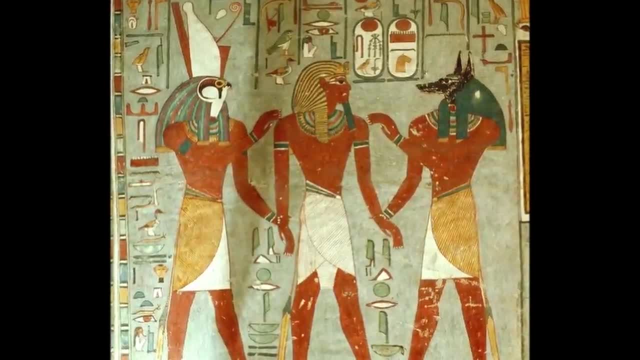 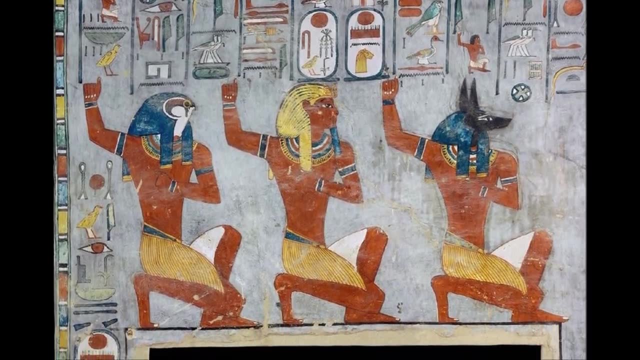 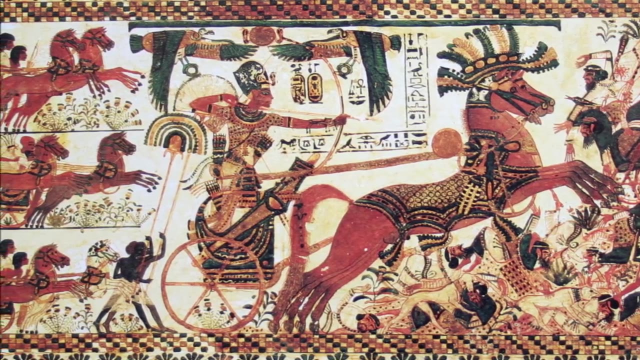 be gods on earth, the sons and daughters of the other gods. It was the job of a pharaoh to keep things in balance and maintain the cosmic order. They would lead armies in battle, collect taxes and build temples to the gods After. 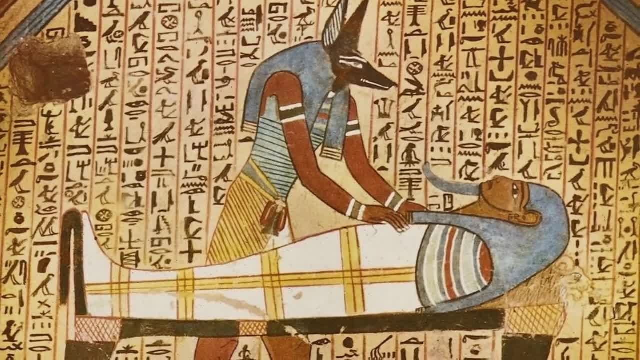 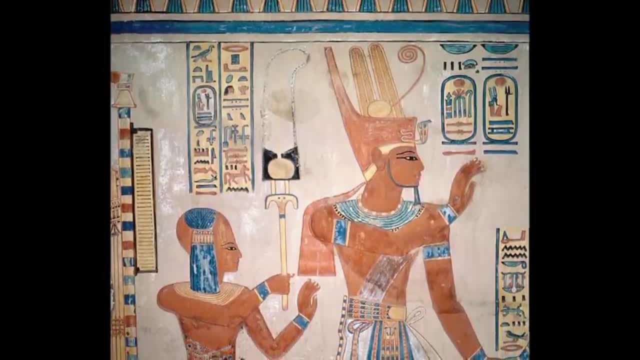 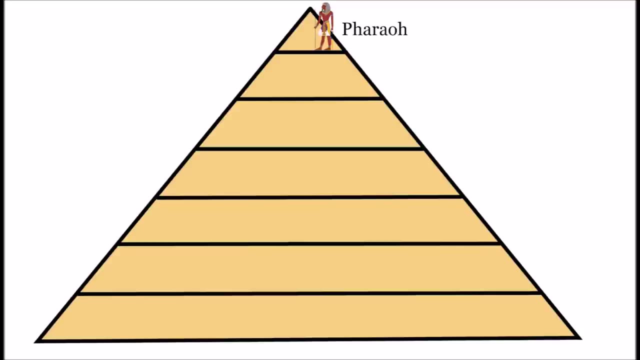 their death. it was believed that the pharaohs would take their place in the afterlife with the other gods, just like Osiris, and leave behind an heir to become the new pharaoh. just like Horus, The pharaoh was the most powerful person in Egyptian society with all the other social 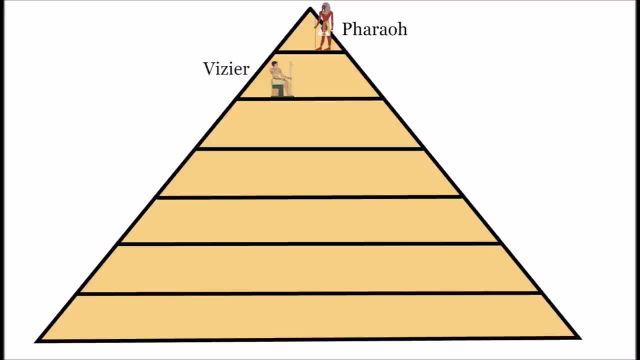 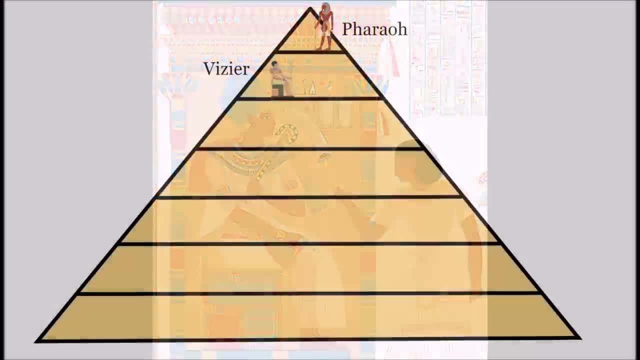 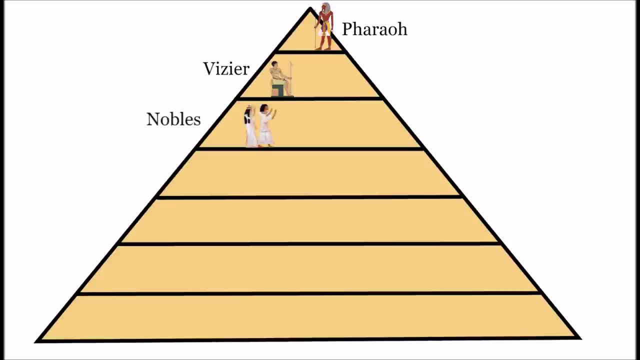 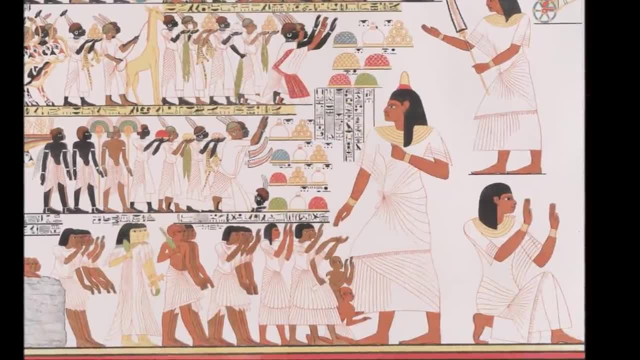 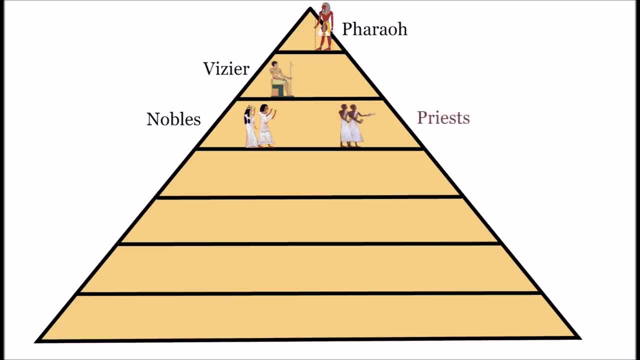 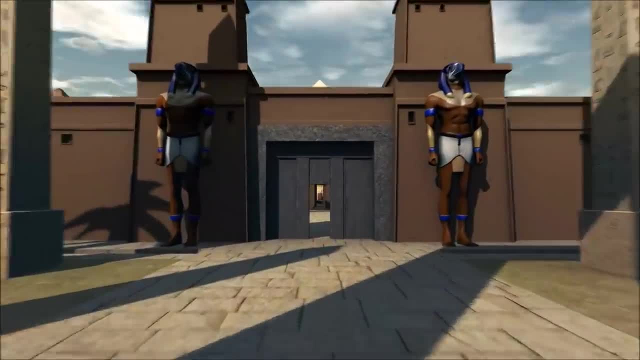 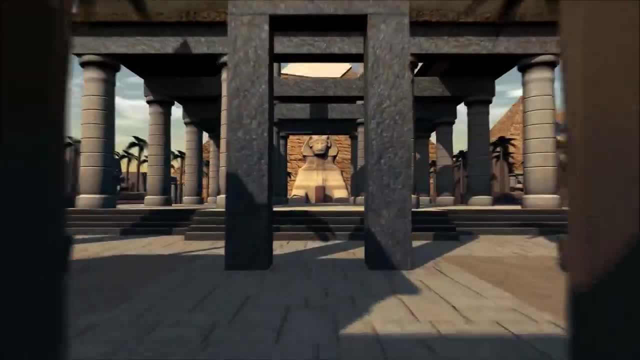 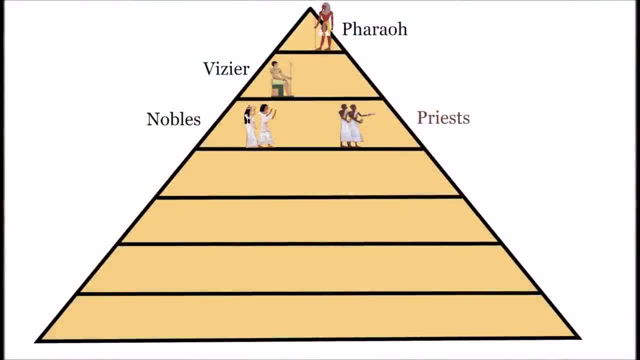 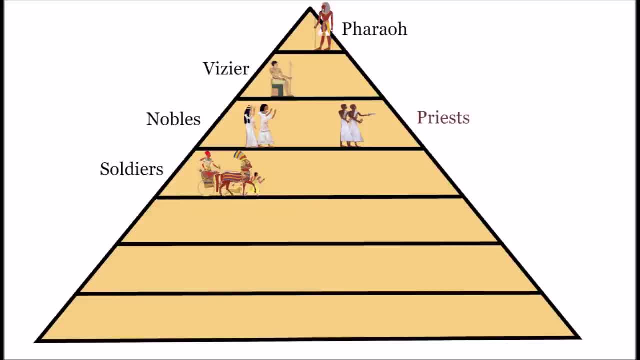 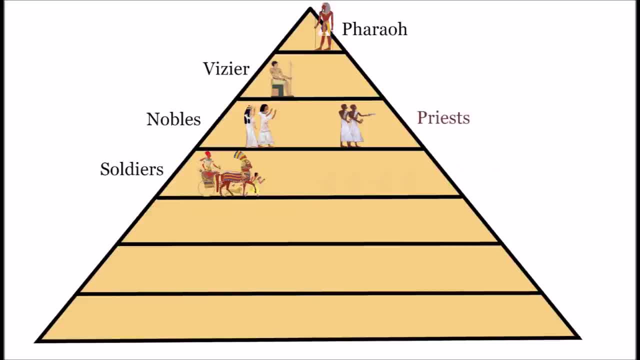 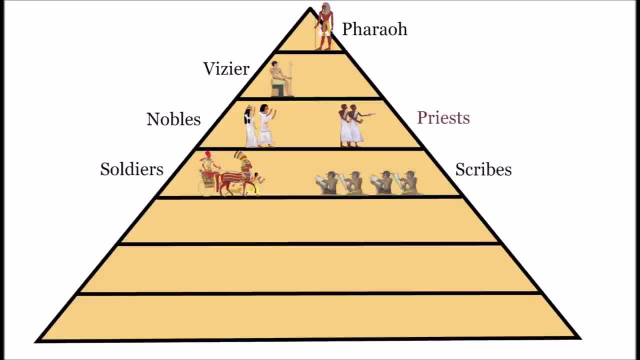 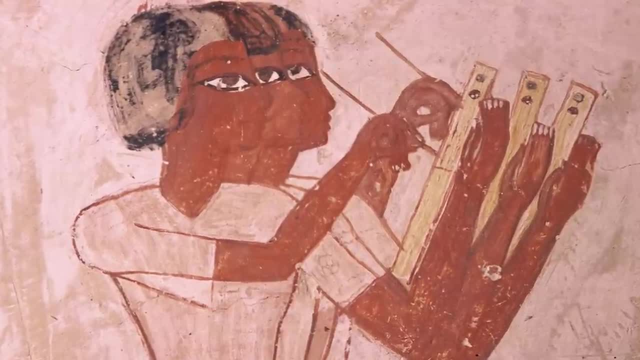 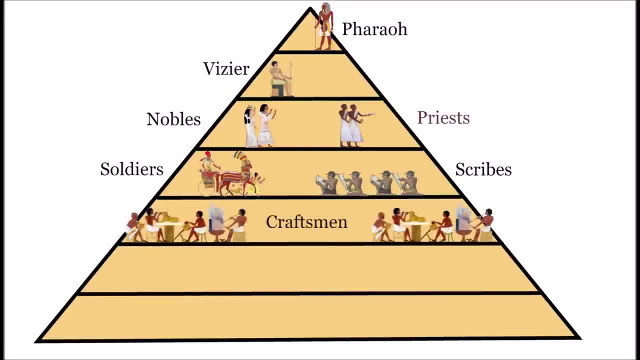 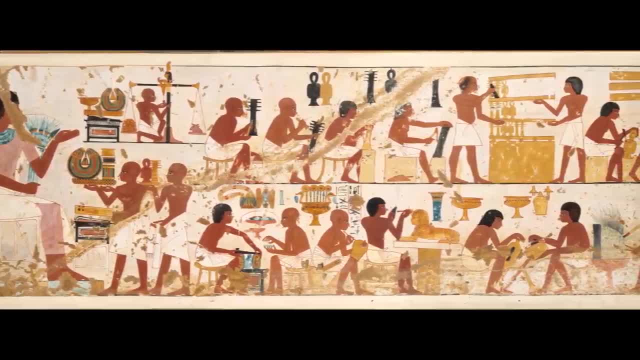 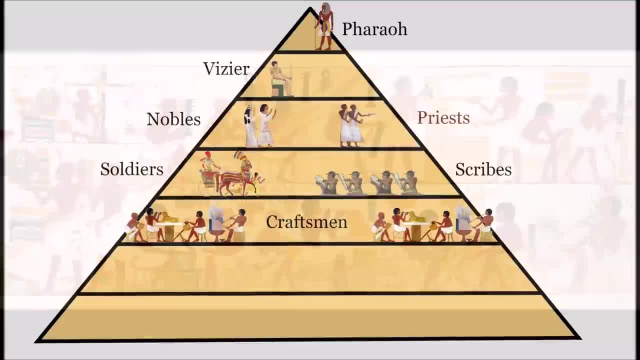 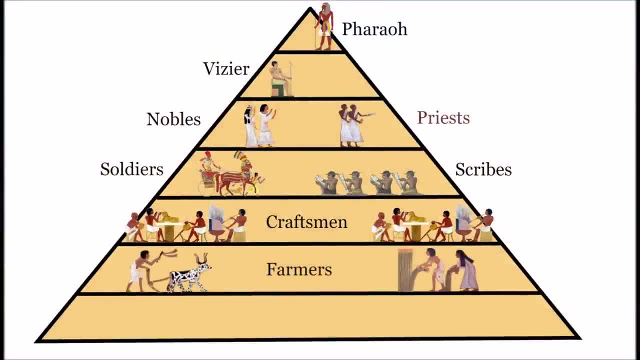 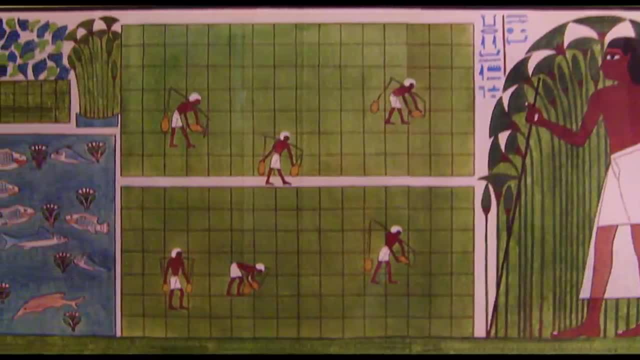 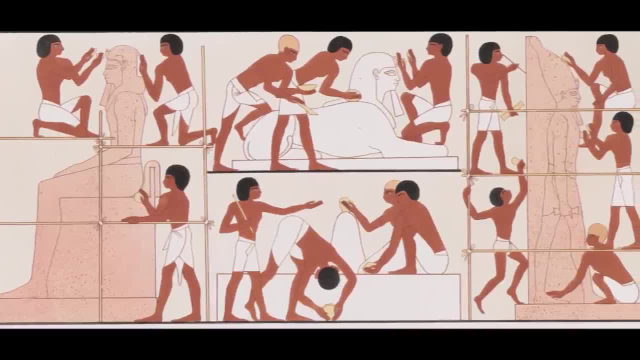 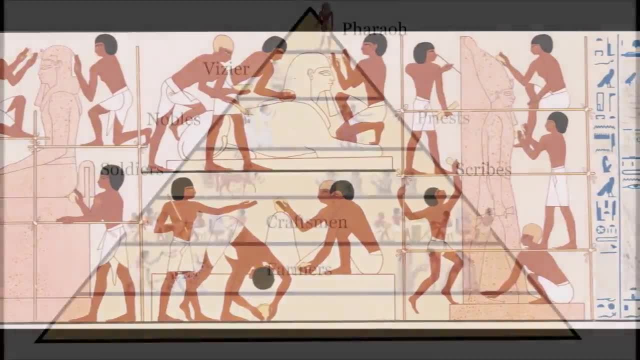 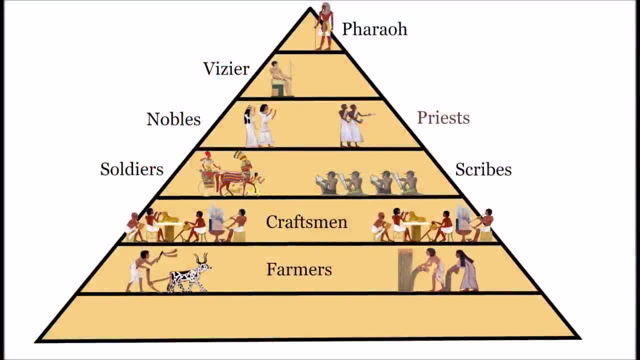 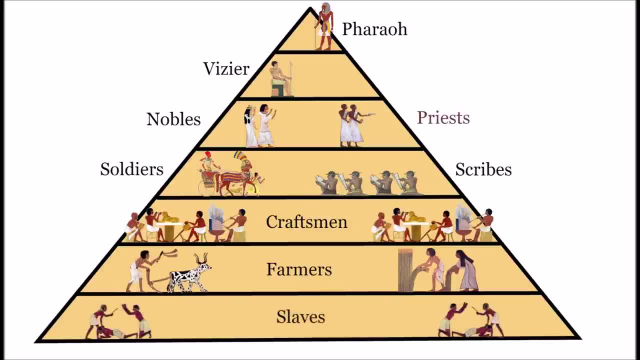 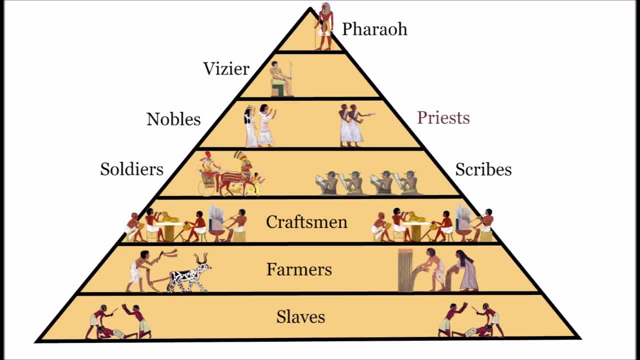 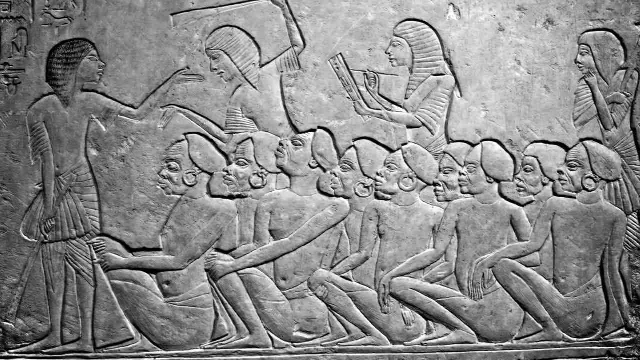 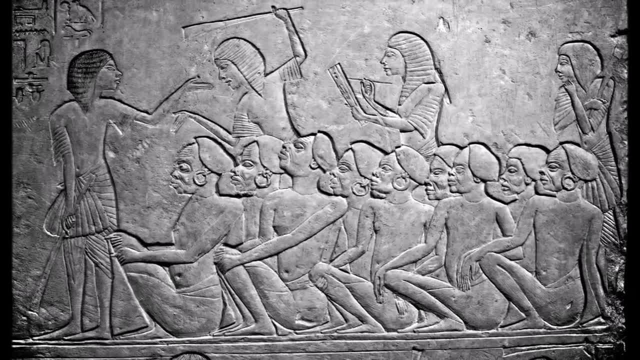 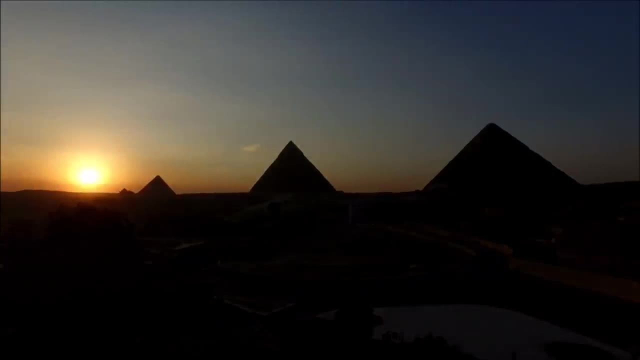 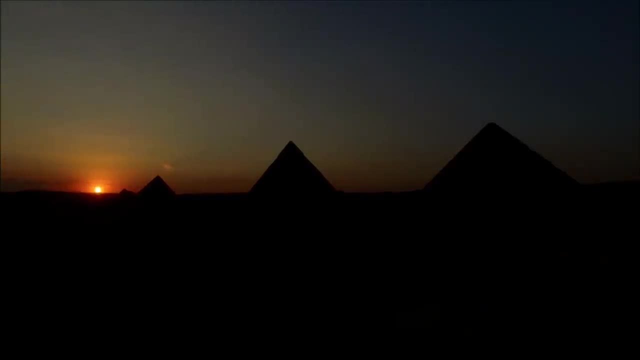 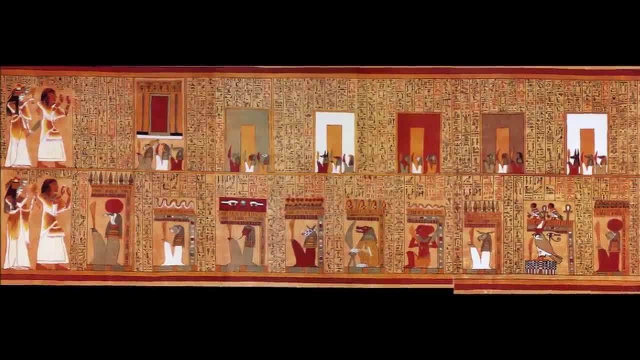 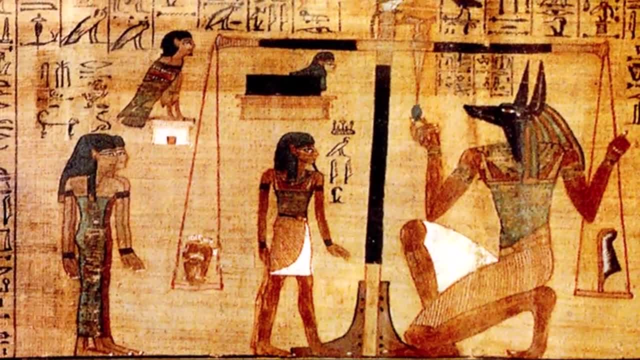 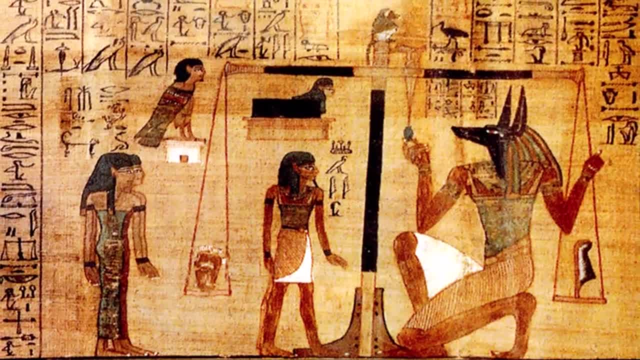 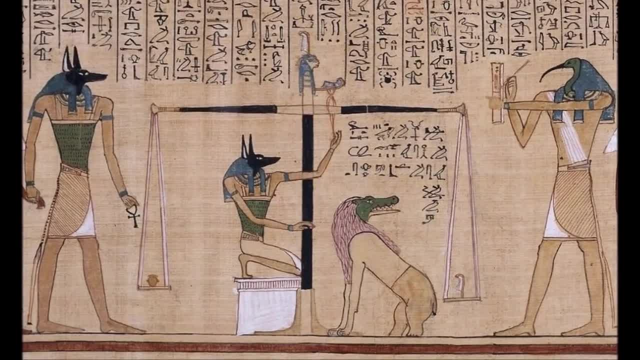 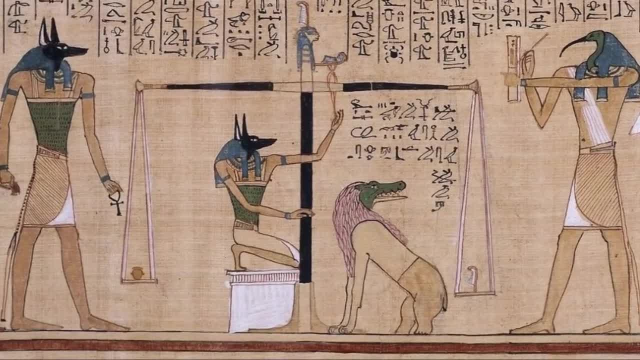 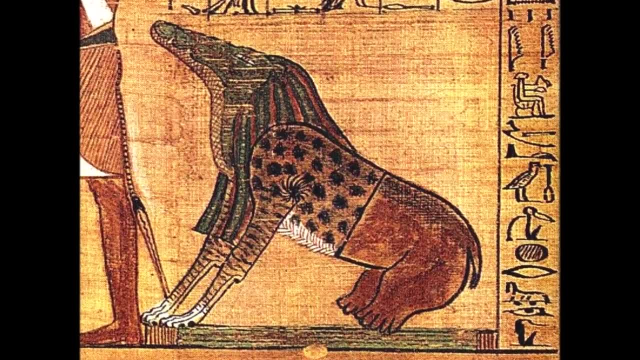 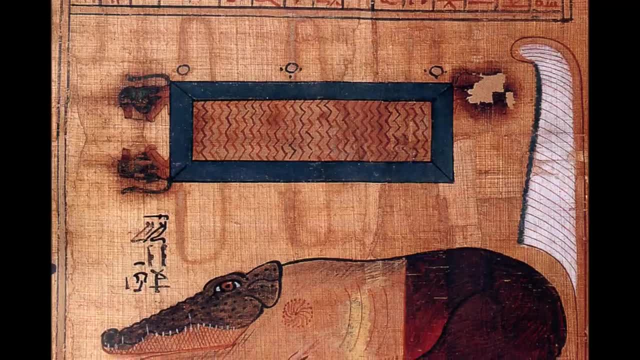 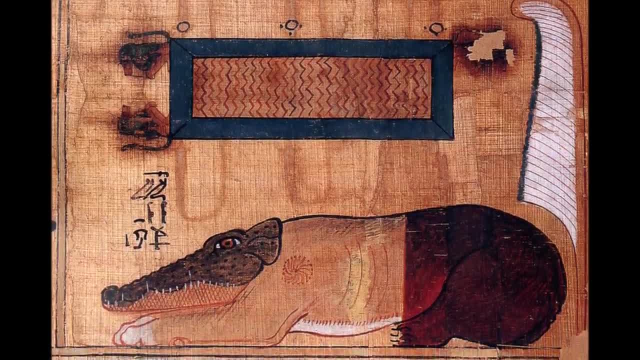 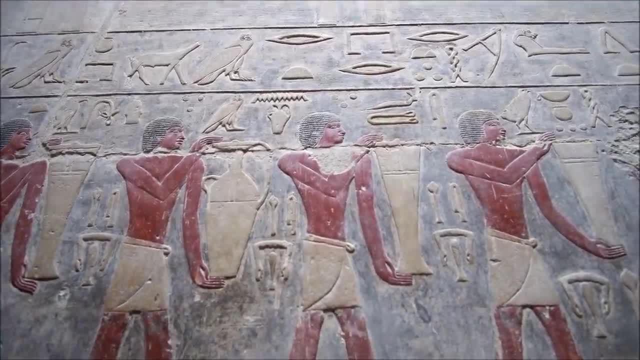 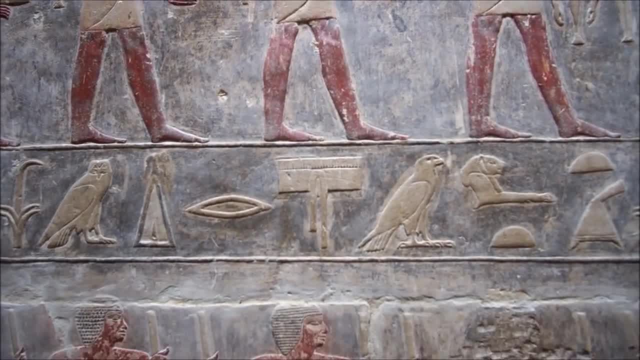 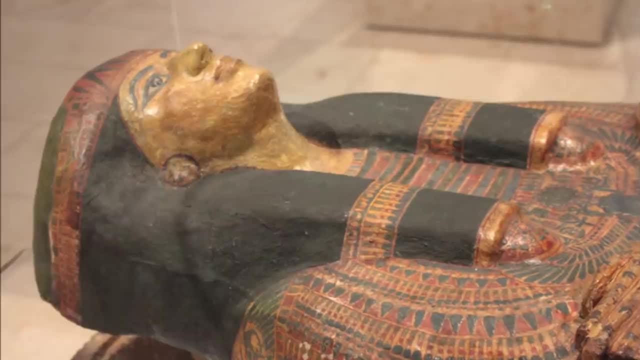 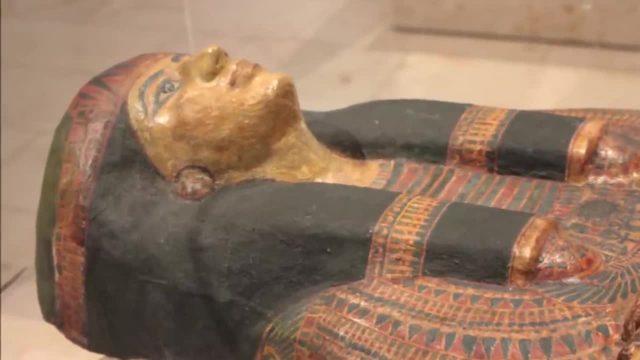 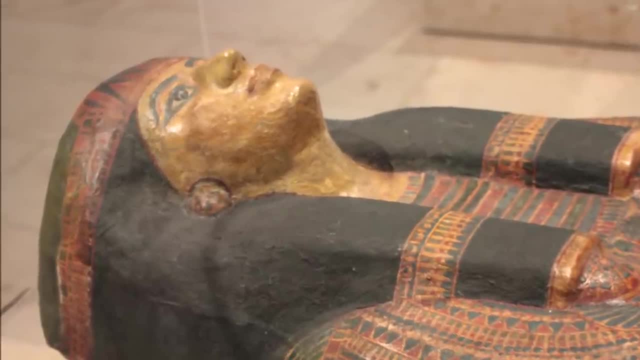 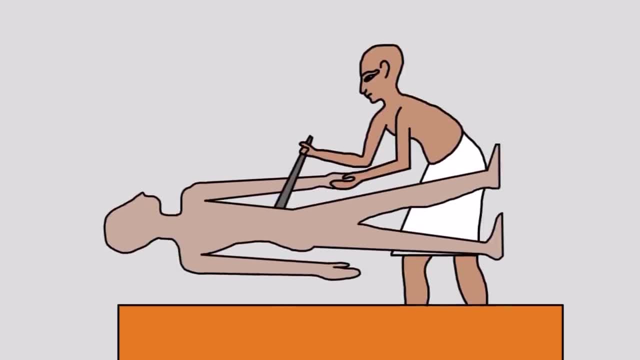 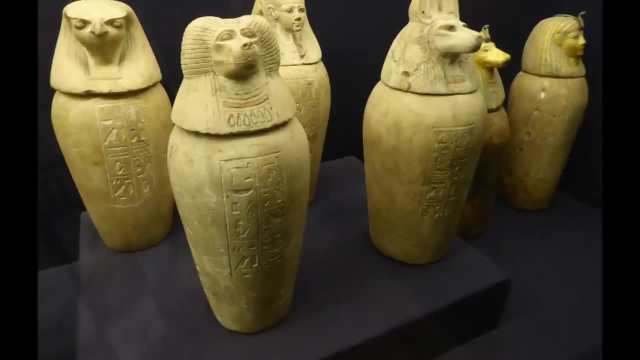 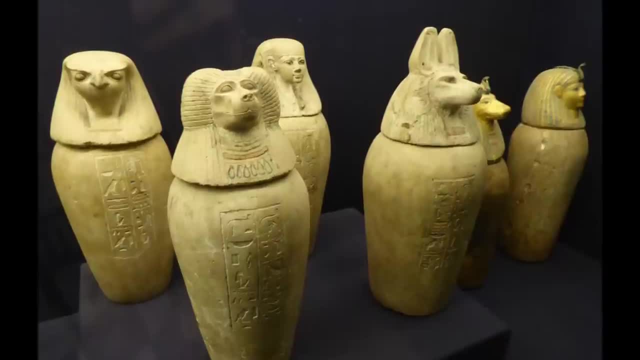 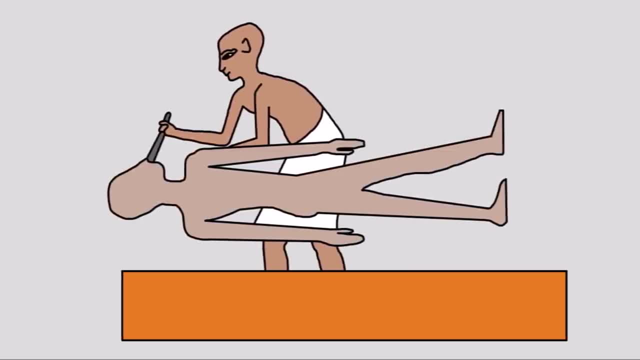 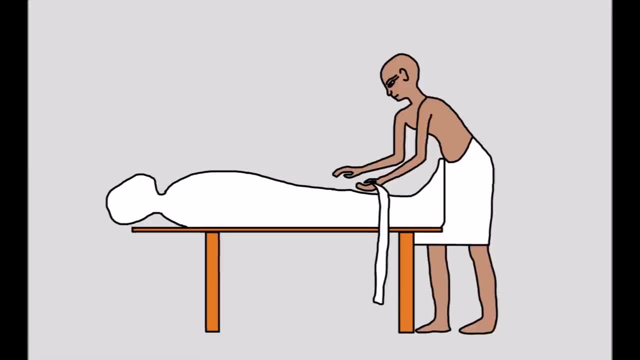 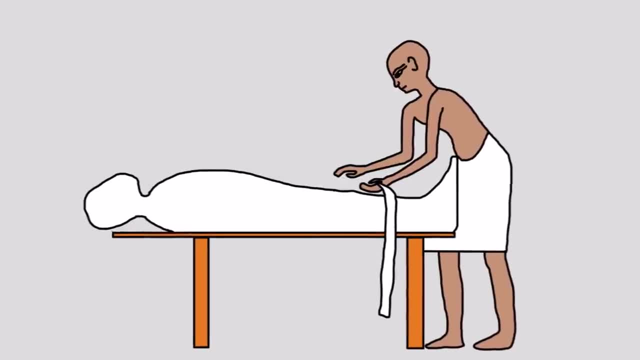 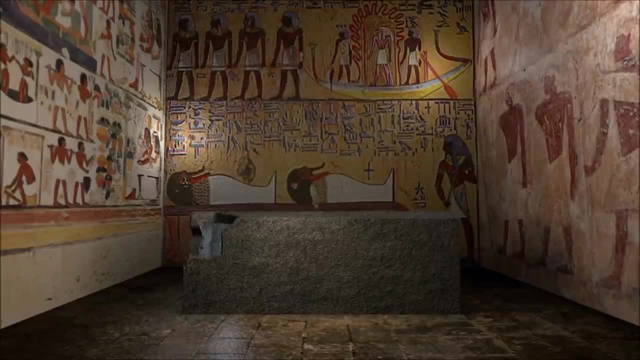 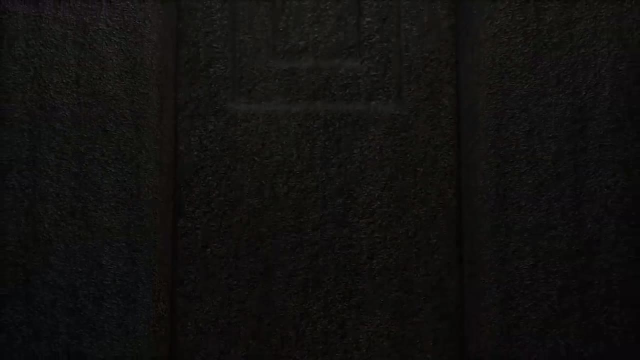 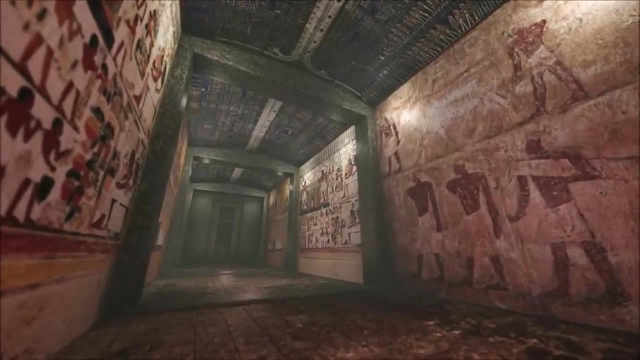 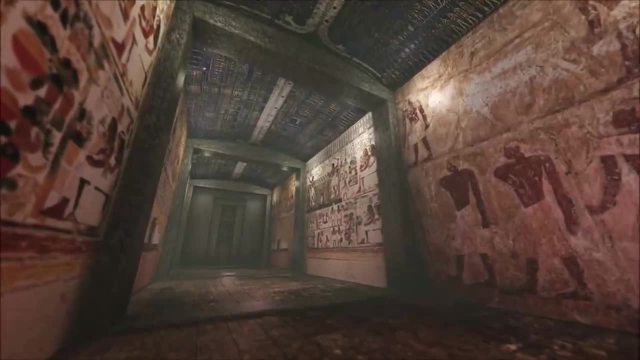 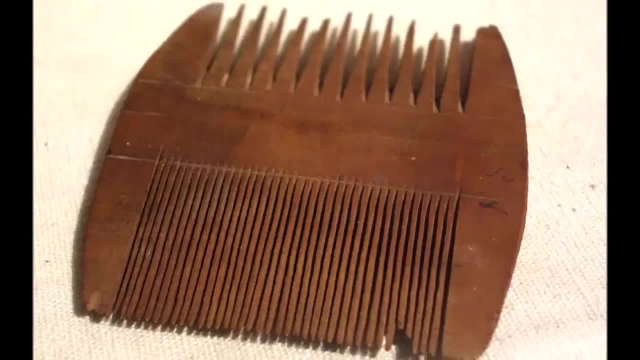 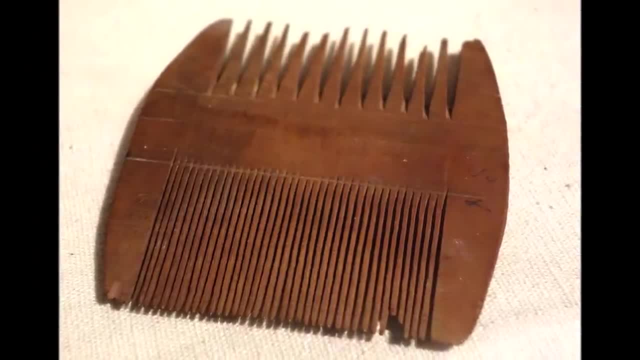 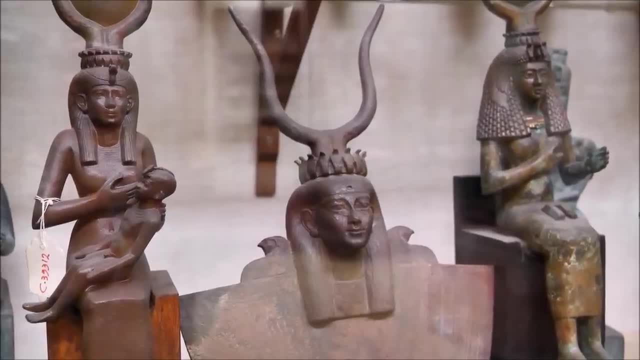 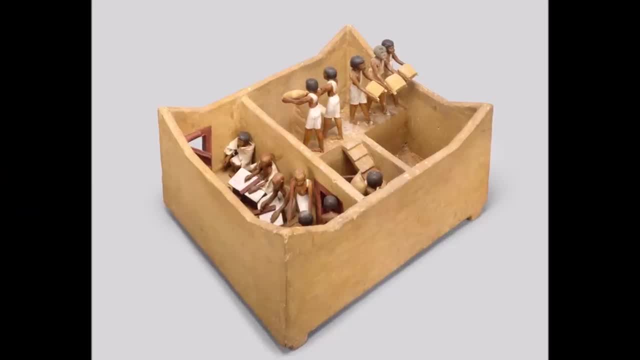 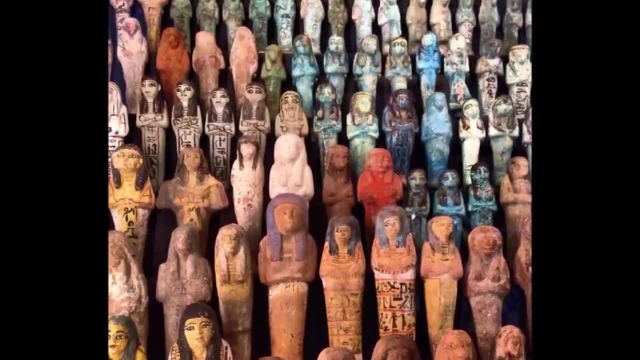 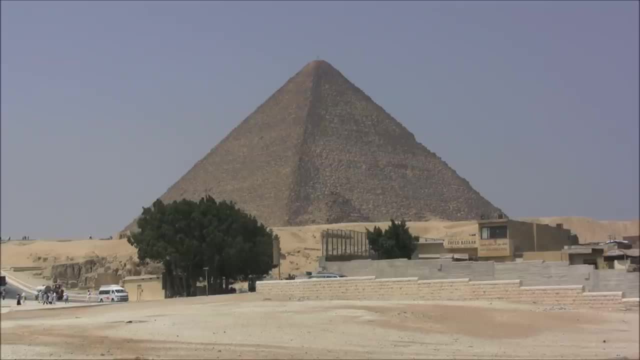 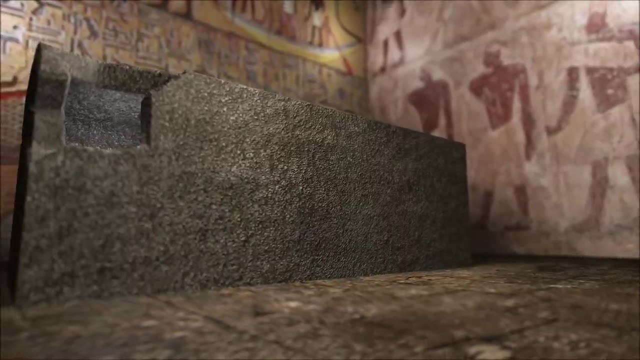 The vizier was the chief of staff in the king's court. The pyramids are examples of tombs that were built for pharaohs to be buried in. There are rooms inside of them where the pharaohs' bodies would be placed, along with any treasures. 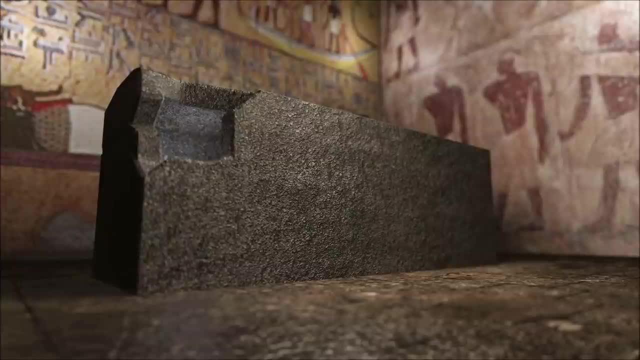 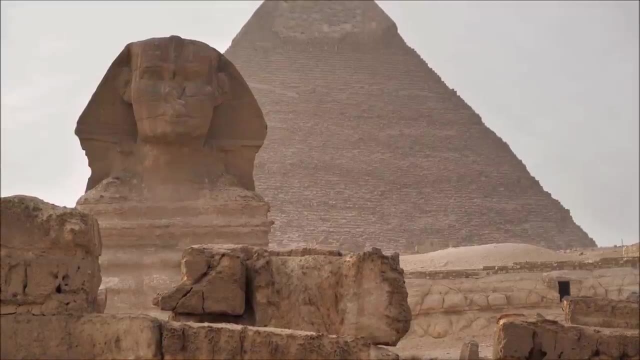 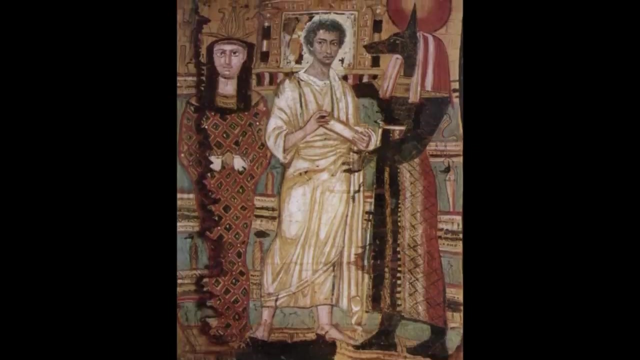 or items that the pharaohs wanted to take with them to the afterlife. Unfortunately, the treasures of most pyramids were stolen long ago, leaving the pyramids empty. About 2,000 years ago, Egypt was conquered by the Romans.